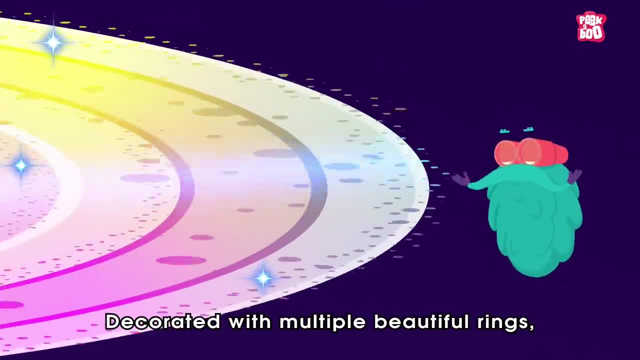 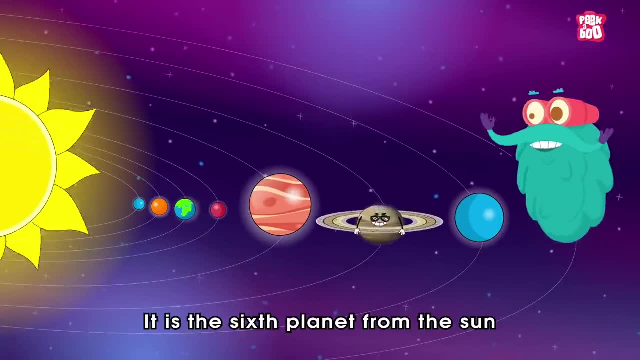 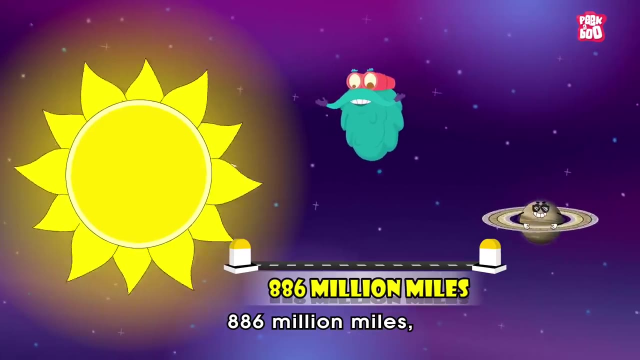 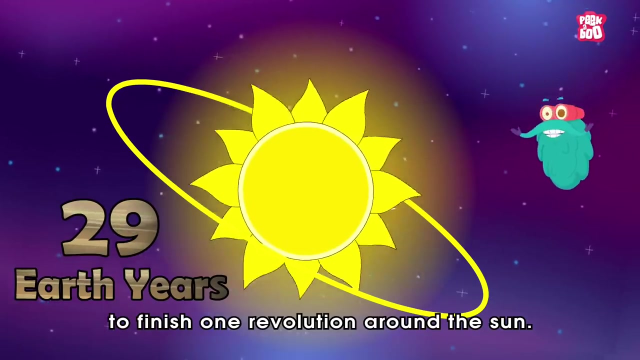 Zoom in. Decorated with multiple beautiful rings, Saturn looks unique among the planets in our solar system. It is the sixth planet from the Sun and orbits at a distance of about 886 million miles, Which takes 29 Earth years to finish one revolution around the Sun. 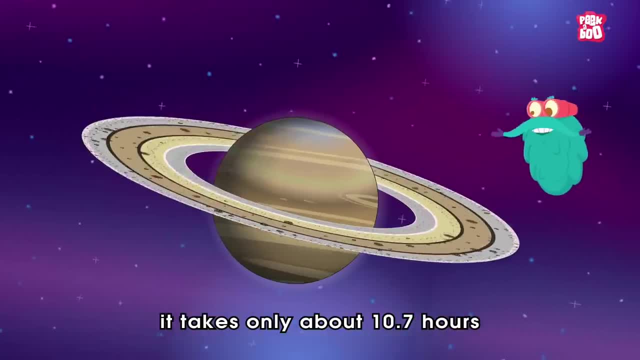 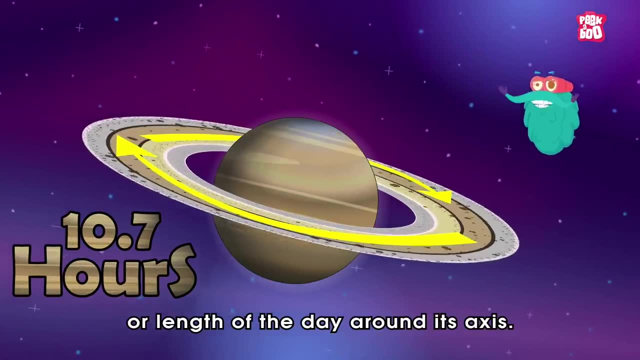 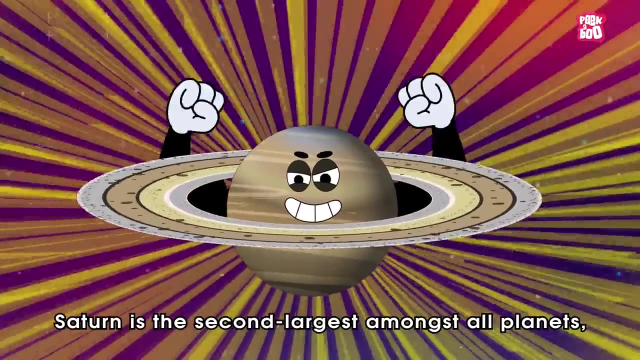 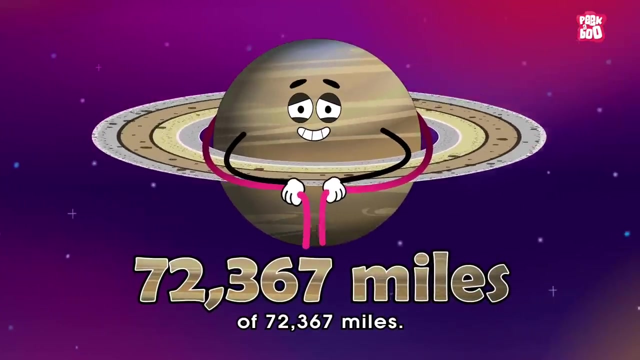 But at the same time, it takes only about 10.7 hours to complete one rotation The length of the day around its axis. In terms of size, Saturn is the second largest amongst all planets, With an equatorial diameter of 72,367 miles. 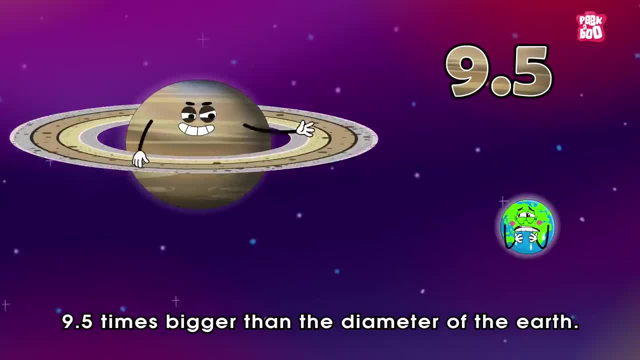 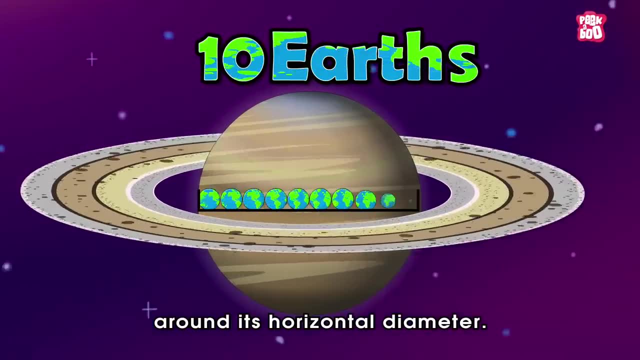 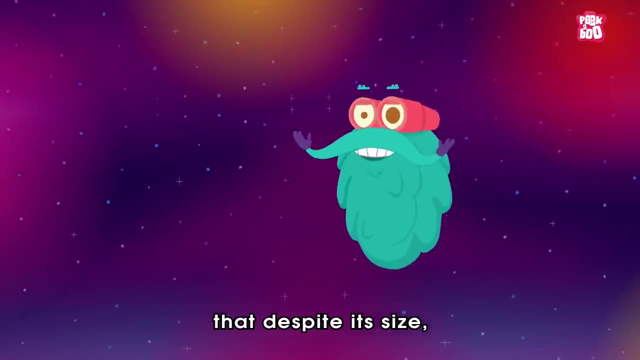 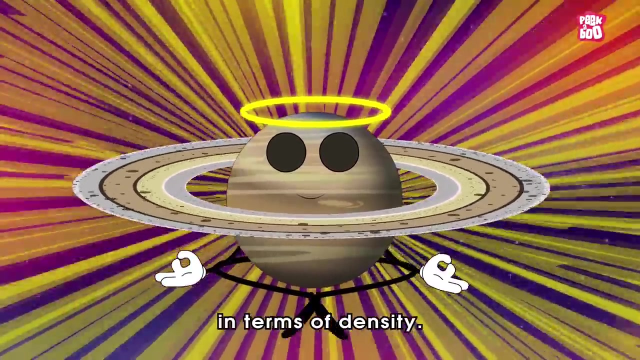 Making it about 9.5 times bigger than the diameter of the Earth. In other words, we can fit around 10 Earths around its horizontal diameter. But you'll be literally shocked to know that, despite its size, Saturn is actually the lightest planet amongst its peers in terms of density. 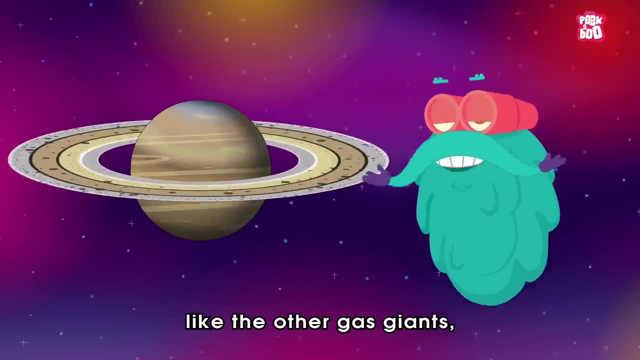 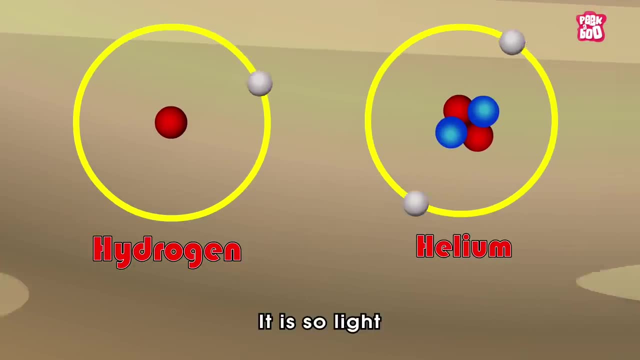 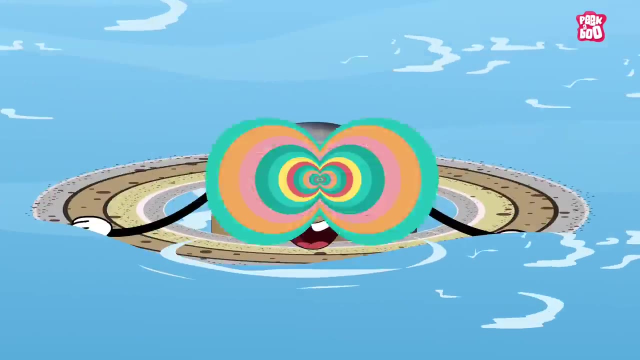 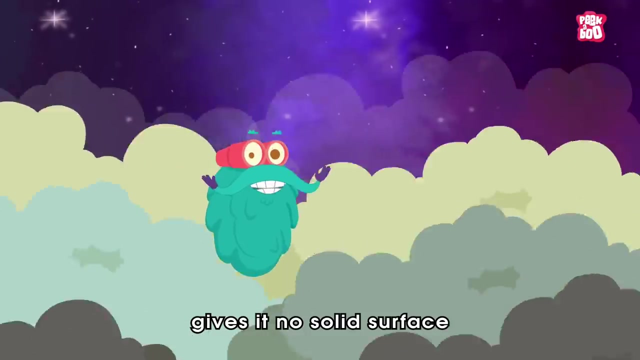 Yes, that's because, like the other gas giants, Saturn is mostly a massive ball of hydrogen and helium. It is so light that it would float in water if there was an ocean big enough to hold it. Not only that, Saturn's gaseous composition gives it no solid surface like Earth. 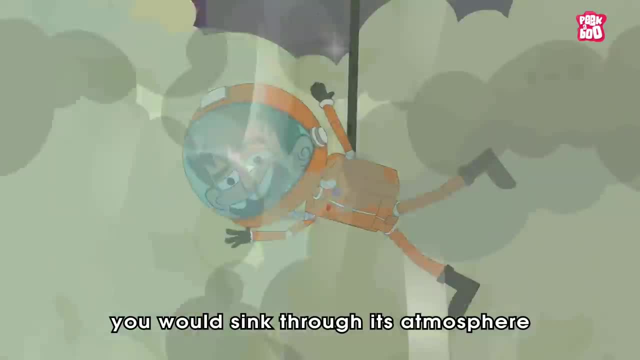 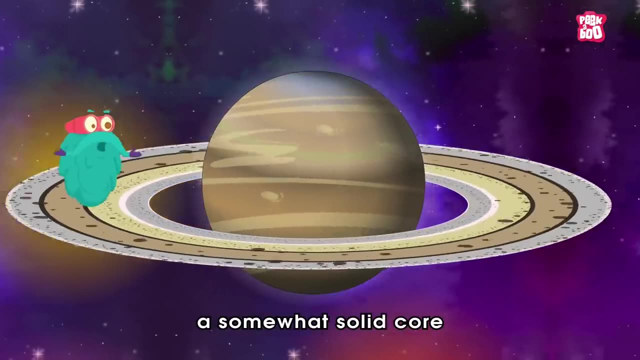 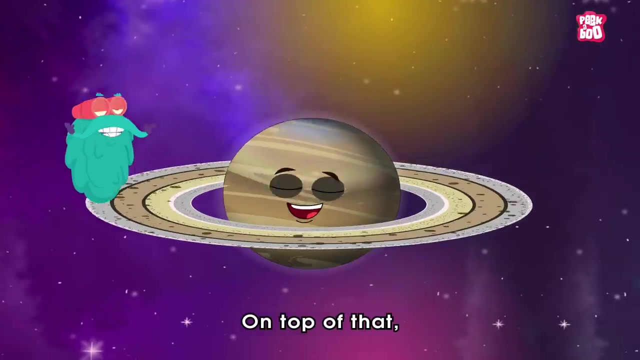 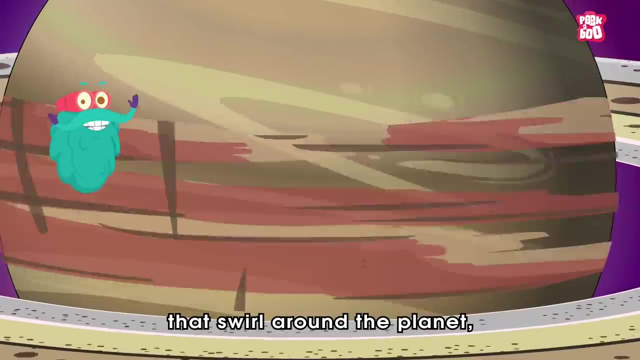 So if you try to walk on it, you would sink through its atmosphere due to air pressure, But it is assumed to have a somewhat solid core Made of rocky material, ice and water. On top of that, the planet is full of gaseous liquid and ammonia crystals that swirl around the planet, causing massive storms. 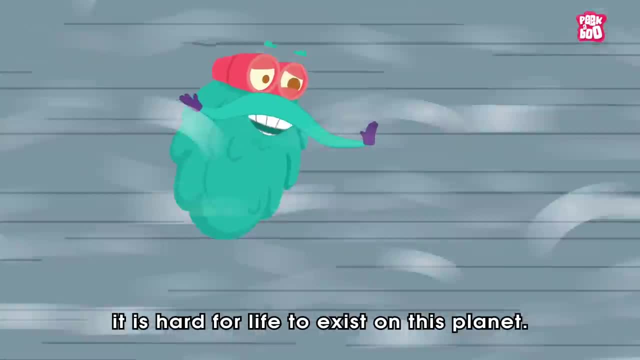 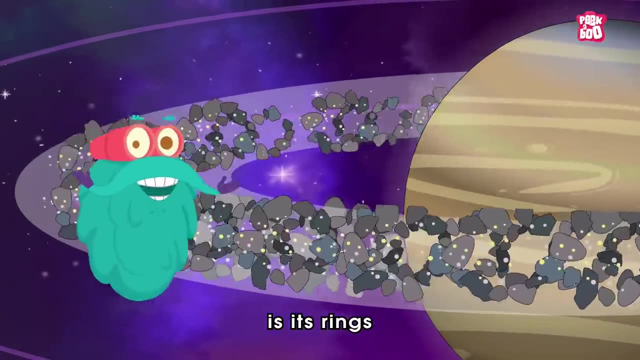 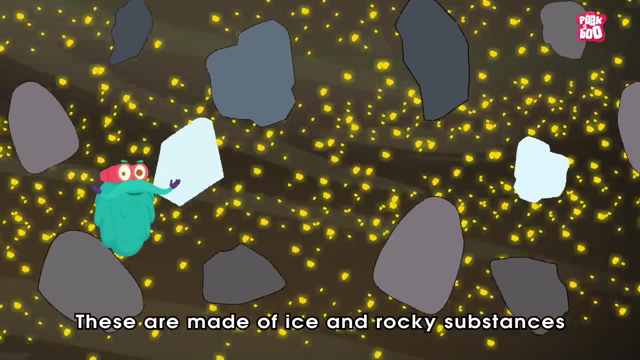 Because of this, it is hard for life to exist on this planet. But what fascinates us the most about Saturn is its rings Extending hundreds of thousands of kilometers from it. These are made of ice and rocky substances that come in various sizes. 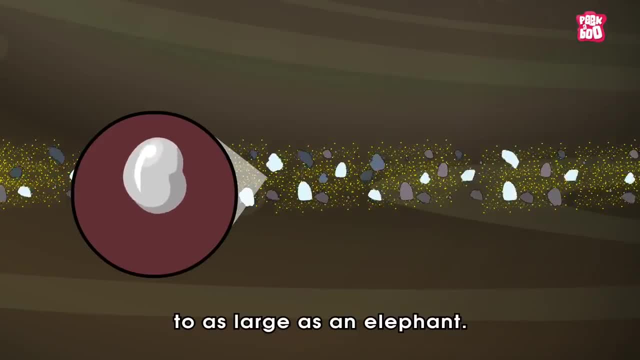 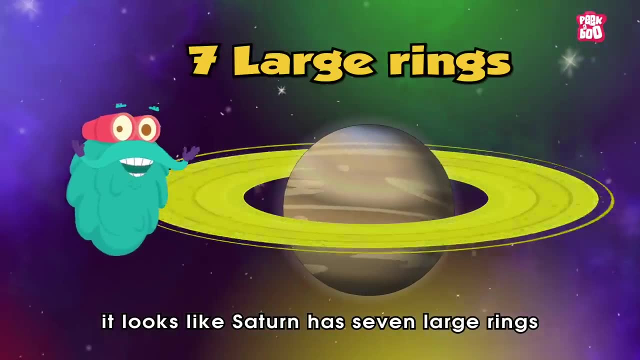 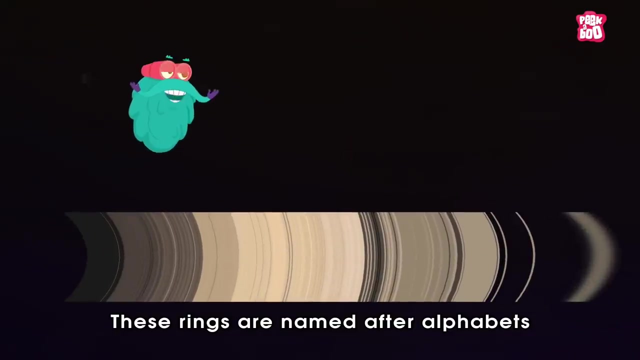 Ranging from a grain of sand to as large as an elephant. From a distance, it looks like Saturn has seven large rings that are separated by gaps called divisions. These rings are named after Allah. They have the alphabets A to G, in the order they were discovered. 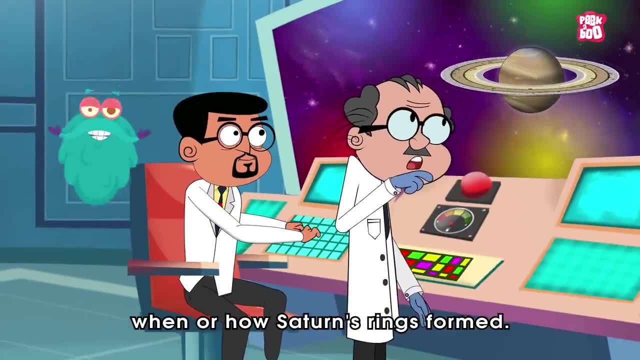 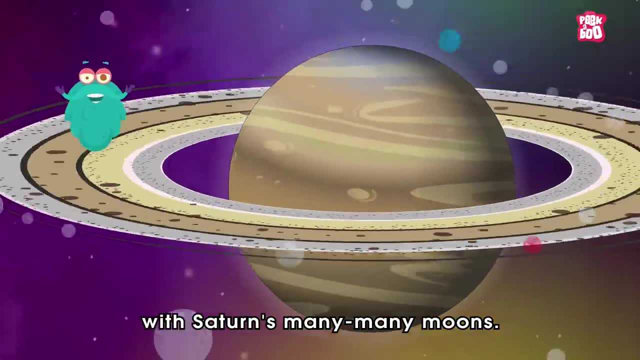 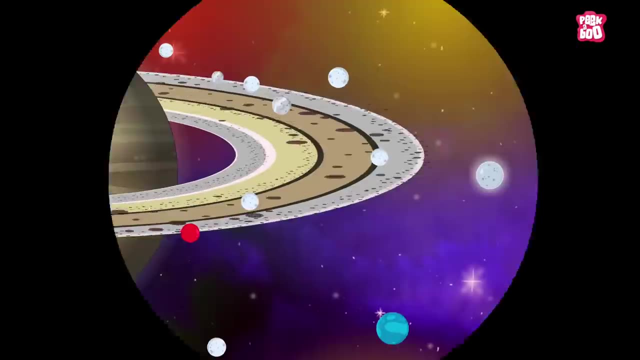 Though scientists aren't sure when or how Saturn's rings formed, However, they assume the rings might have something to do with Saturn's many, many moons. Yes, unlike Earth's one and only moon, Saturn has at least 53 known moons. 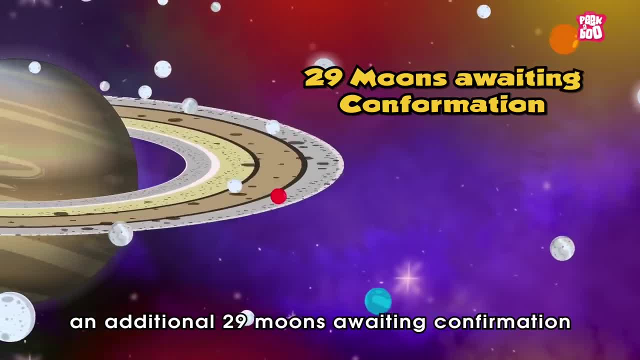 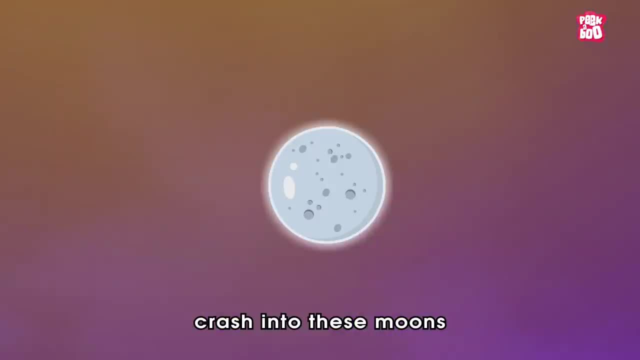 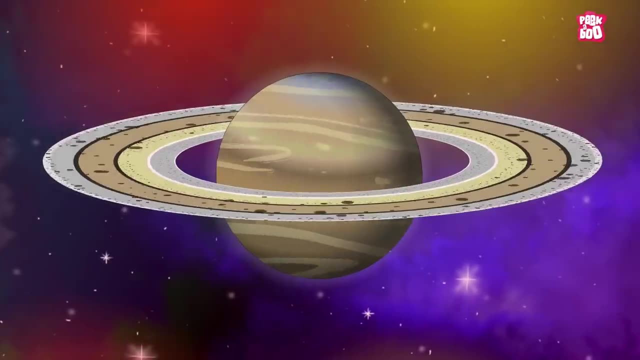 With an additional 29 moons. These moons are waiting confirmation of their discovery. So at times, asteroids and meteoroids crash into these moons and break them into pieces, Forming the iconic ring structure, Which is as wide as four and a half Earth. 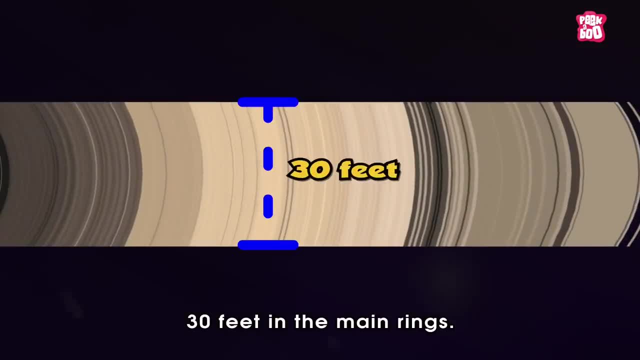 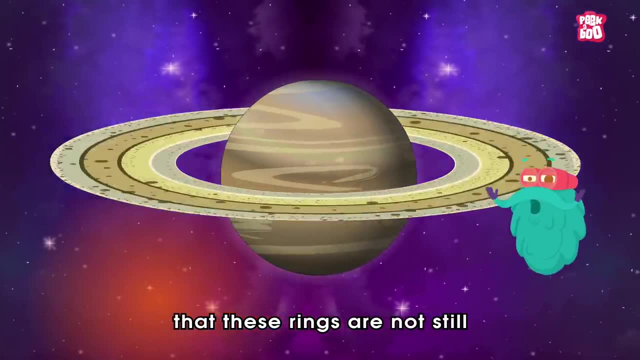 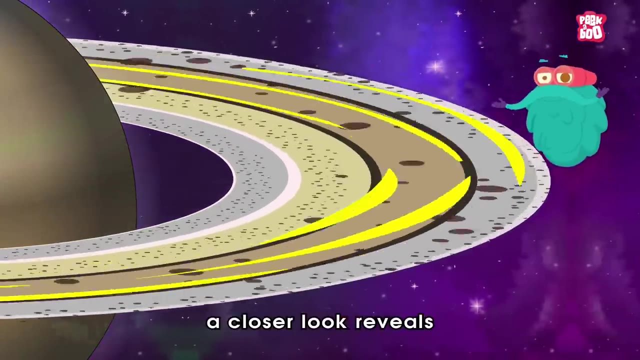 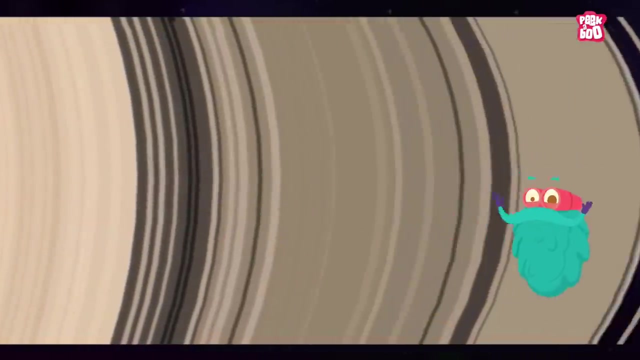 Yet the vertical height is only about 30 feet in the main rings, And you will be amazed to know that these rings are not still, but circle around Saturn at very high speeds. Not only that, a closer look reveals that each large ring is made up of many small rings, sometimes called ringlets. 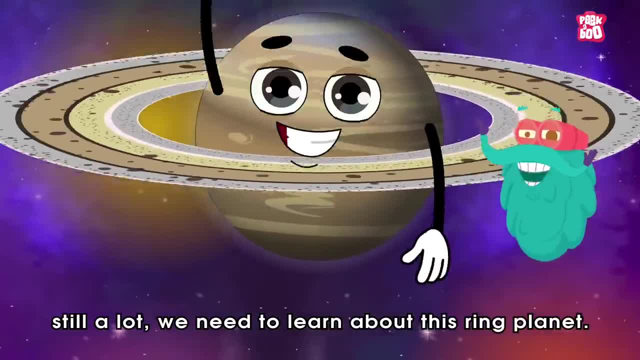 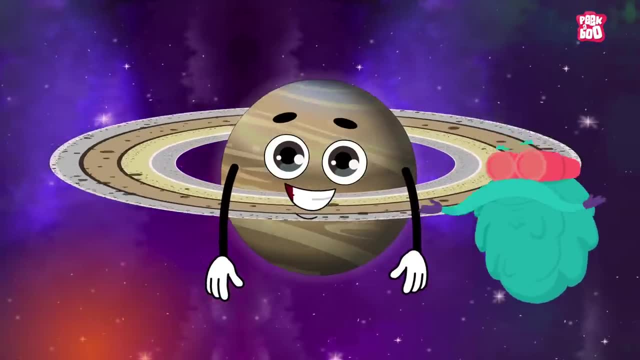 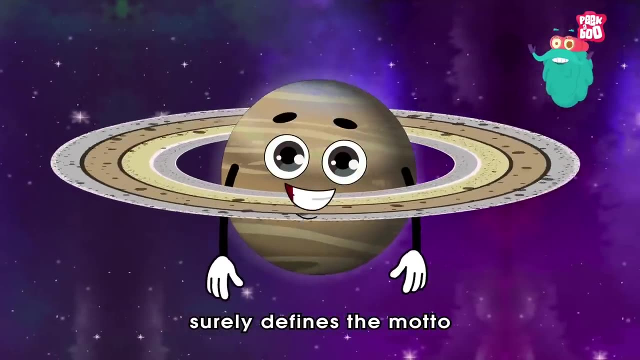 Though there is still a lot we need to learn about this ring planet. However, whatever we know, we can surely say that Saturn, with its many moons, multiple rings and gassy composition, Surely defines the motto: be different better than anything else in the known universe. 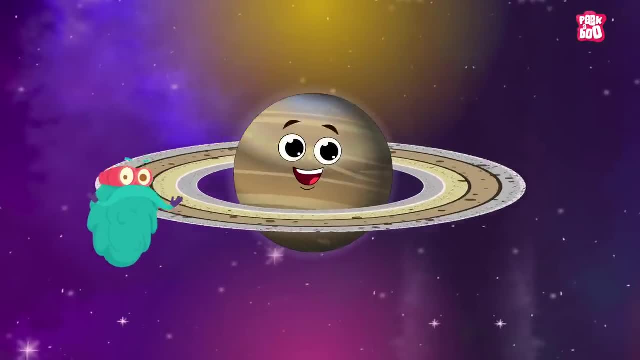 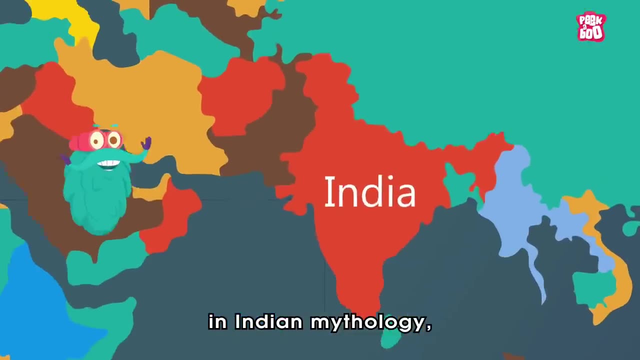 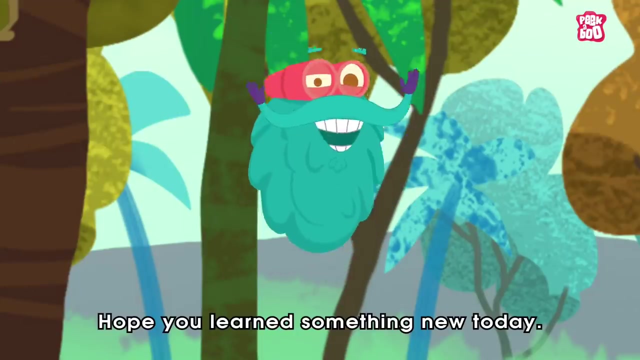 Trivia time. Did you know Saturn is named after the Roman god Saturnus, Whereas in Indian mythology Saturn is often called the god of justice. Hope you learnt something new today, Until next time. it's me DrBinox zooming out. Transcription by ESO. translation by —.